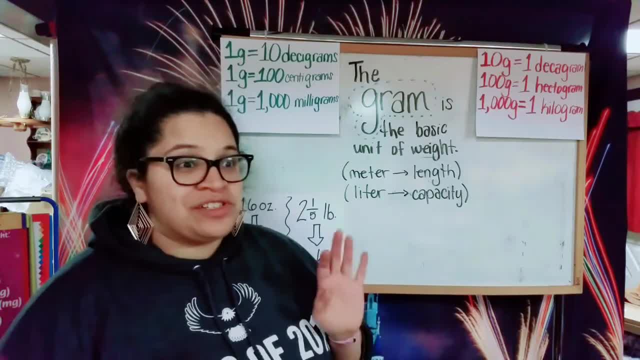 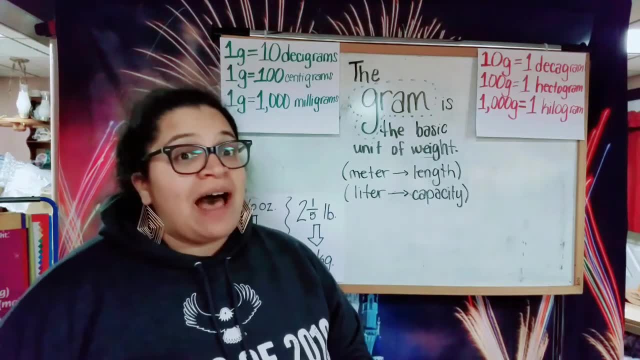 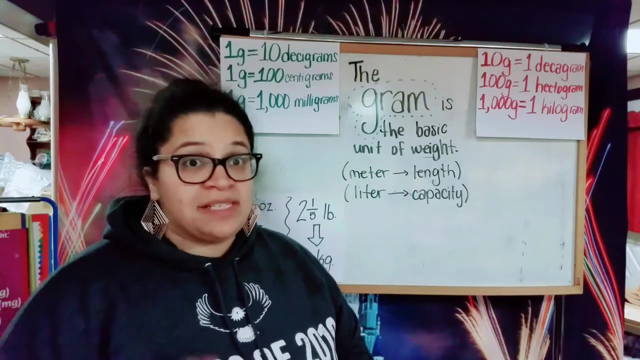 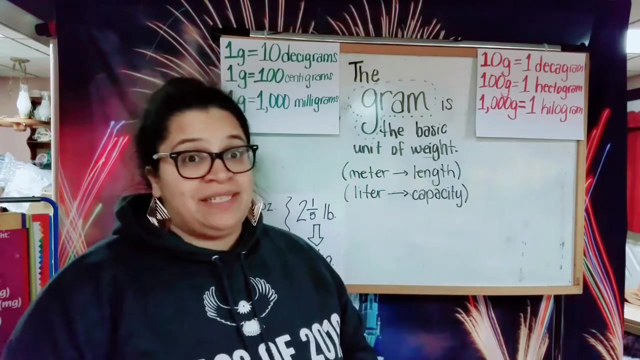 Versus our standard English system of measure, which is just all sorts of complicating crazy. So if you're a little unfamiliar or need a refresher on the metric prefixes, there is a video where we practice the prefixes with the flashcards And I will put that link in the description box of this video. But let's go ahead and let's talk about the different measures of weight, Because a gram can be broken up into smaller pieces and larger pieces. 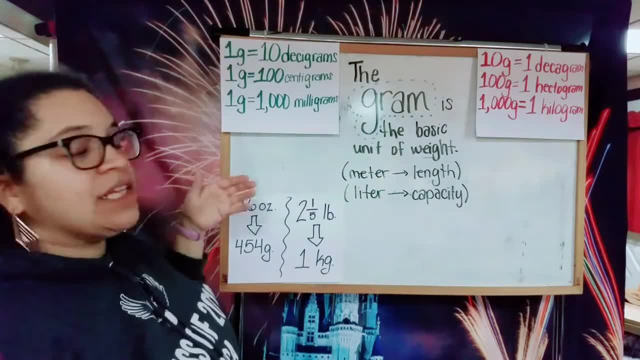 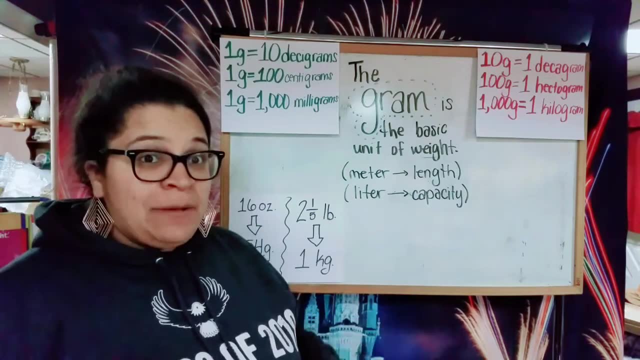 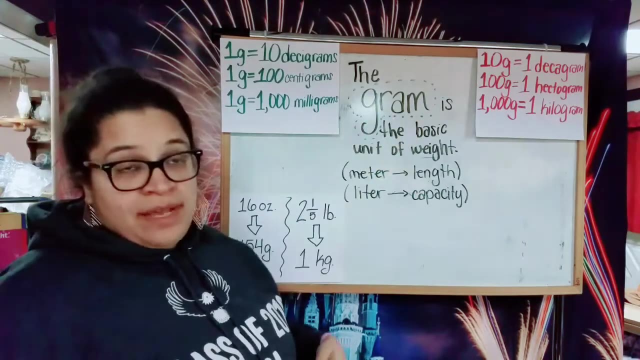 And so here to the left of the gram, I have the smaller units. We talked with prefixes about how deci, centi, milli they all end in I. All of those prefixes mean I'm talking about a smaller unit of measure than my basic unit. So these are all smaller. Let's go ahead and hopefully you can read them. okay, Let's go ahead and read these together. 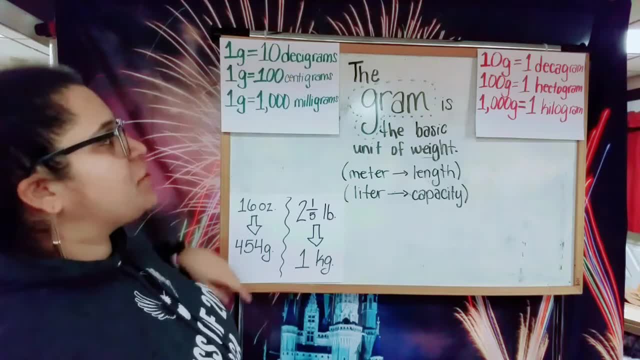 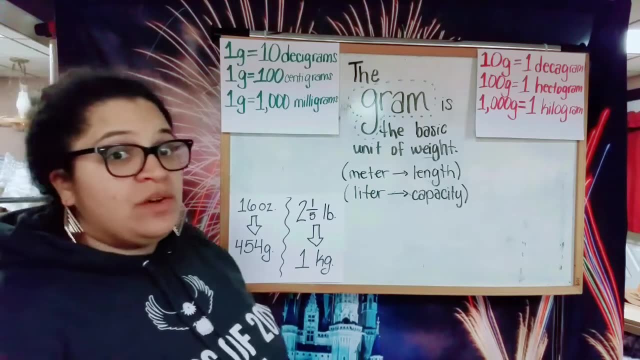 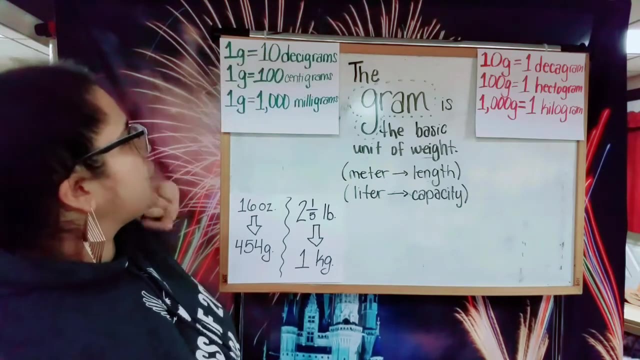 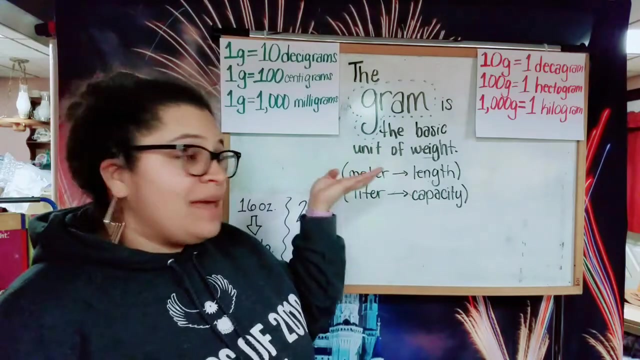 One gram equals ten decigrams. One gram equals one hundred centigrams. One gram equals one thousand milligrams. One more time: One gram equals ten decigrams. One gram equals one hundred centigrams. One gram equals one thousand milligrams. Alright, so those are all of the gram units that are smaller than a gram. Let's talk about the ones that are larger than a gram. 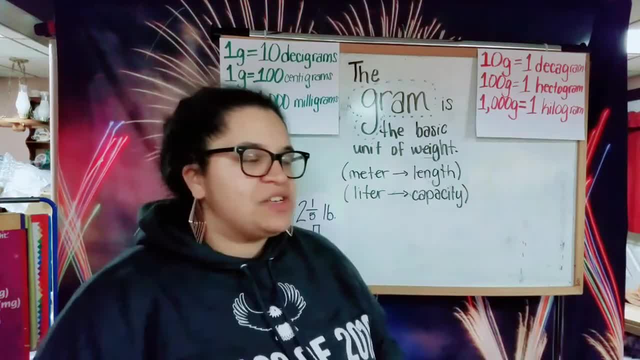 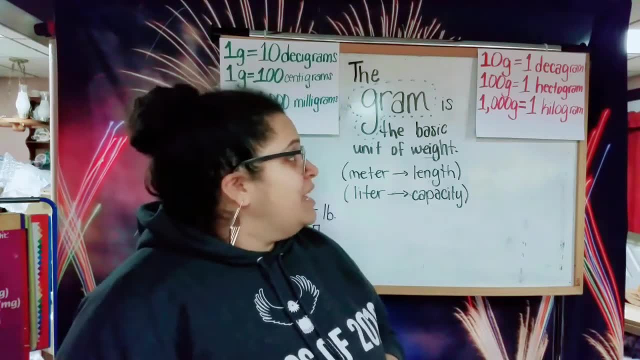 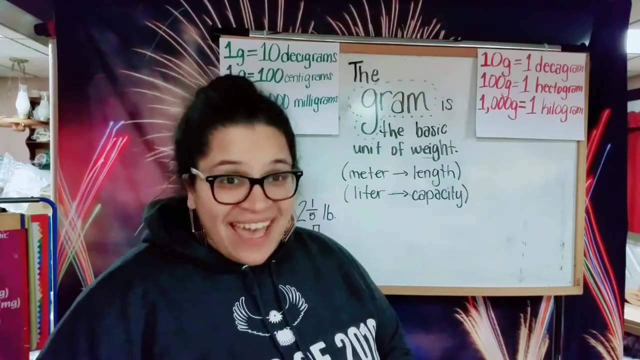 And so again, if you have a basic understanding of Latin prefixes, you'll know that decimals and decimals are the same deca. how many years are in a decade? 10.. And that will hopefully help you a little bit with some of these. And then my trick for a hecto. hecto starts with an H, 100 starts with an H. 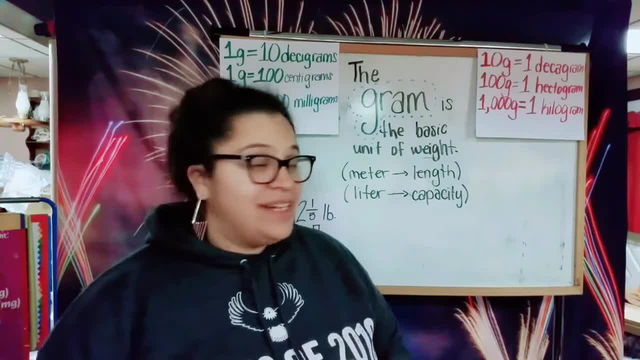 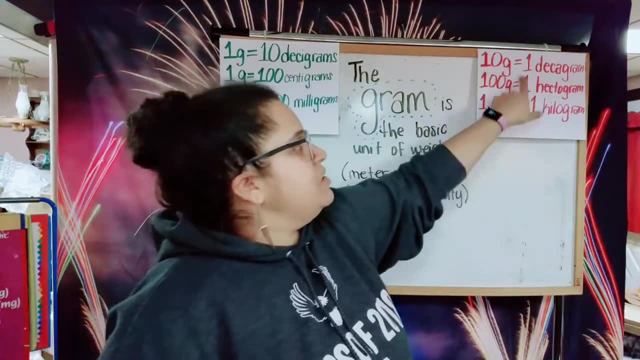 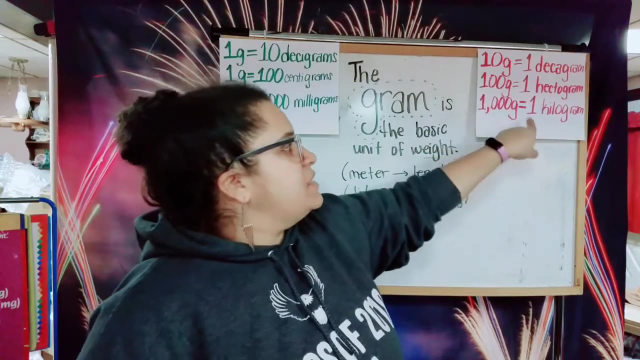 So I like to stress that hecto is 100. And then kilo is just one of those you kind of have to memorize. So here we go. 10 grams equals one decagram. 100 grams equals one hectogram. 1,000 grams equals one kilogram. Let's try those again. 10 grams equals one decagram. 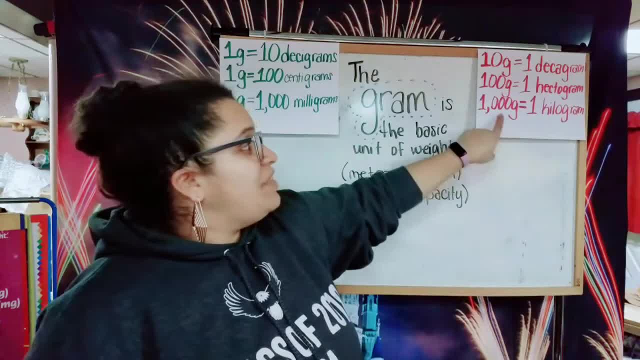 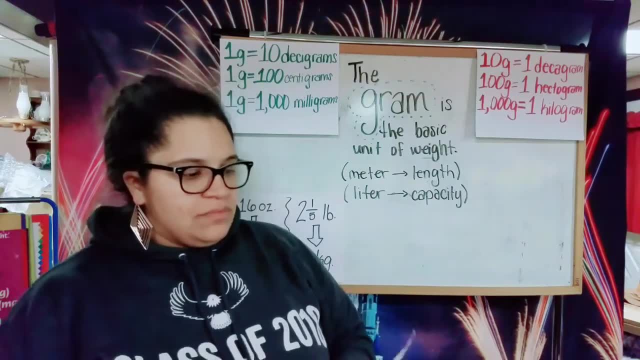 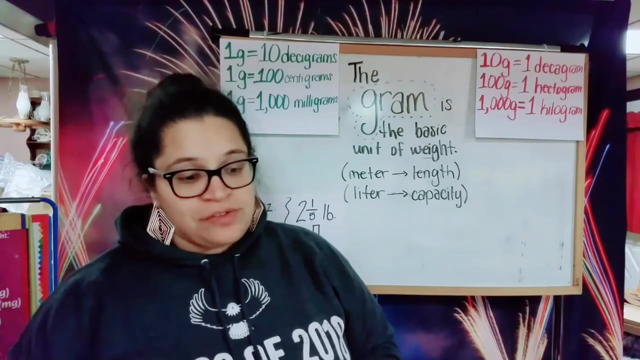 100 grams equals one hectogram. 1,000 grams equals one kilogram, And again the gram is the basic unit of weight. And so again, the gram is actually a very, very small unit. In fact, many items in the grocery store are marked. 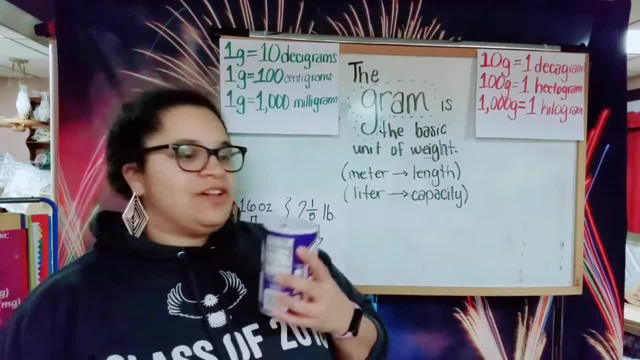 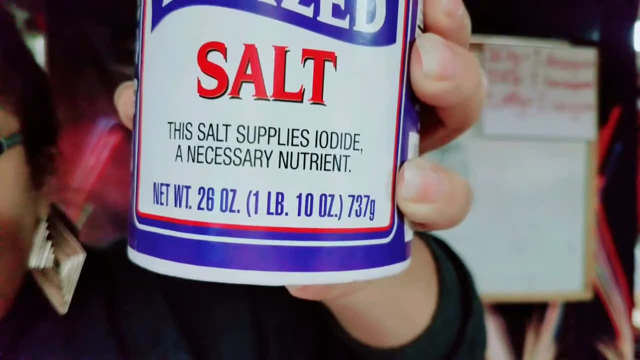 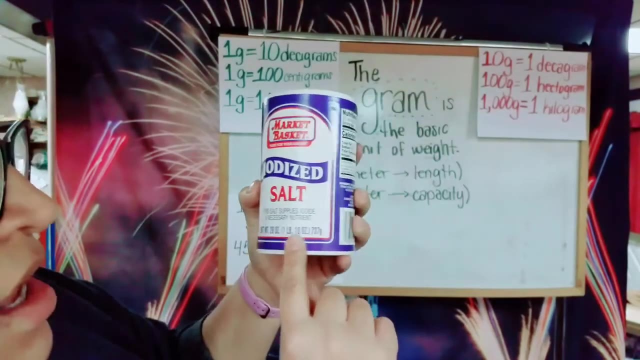 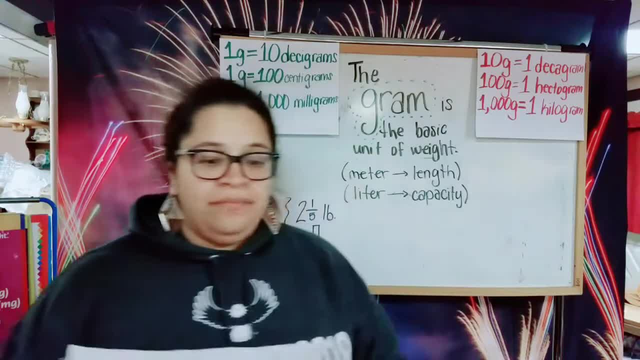 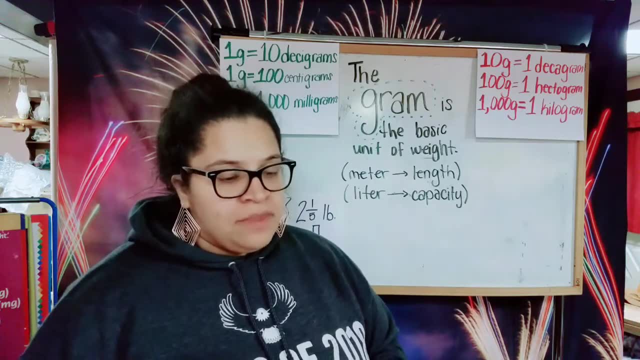 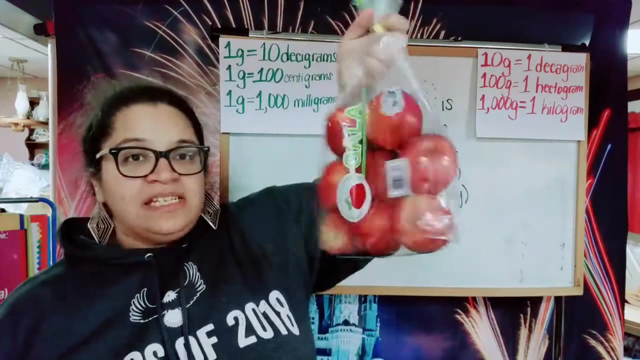 put othe lot of grams in here. A kilogram is the most frequently used measure in the grocery store. A kilogram is about two pounds and three ounces, And so actually one of the easiest ways I use to remember the kilogram is a bag of apples, So that two and one-fifth pounds. 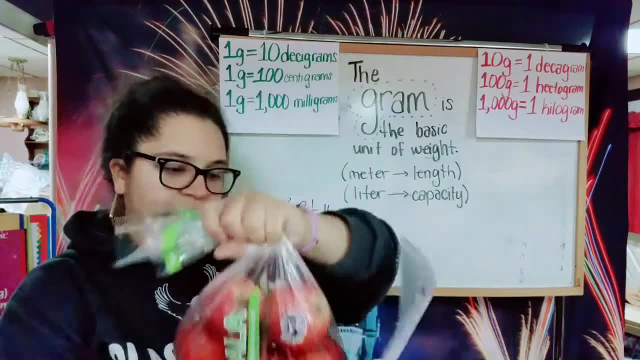 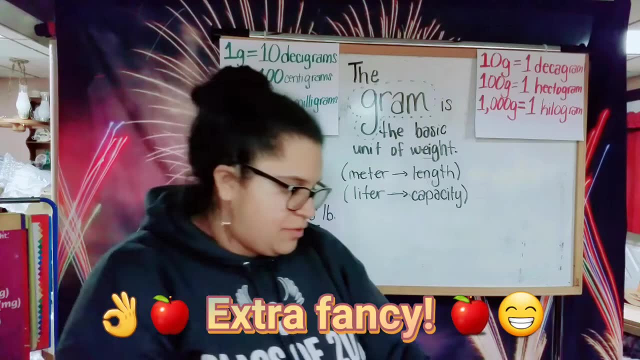 It's about a kilogram of apples And, in fact, my label: these are extra fancy. Thank you, maroga and coolato, for being extra fancy apples. Oh, yes, yes. So this says that this is three pounds of apples. 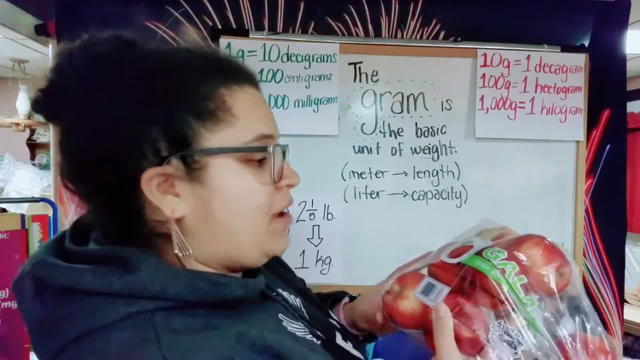 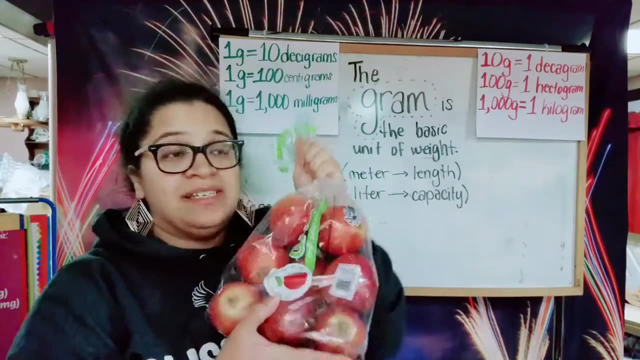 So it's a little bit bigger than two and one-fifth pounds And in fact this is 1.36 kilograms. So a kilogram is roughly a bag of apples. if that helps you remember that weight at all, Next time you're with your grown-up at the grocery store, go ahead and pick up one of 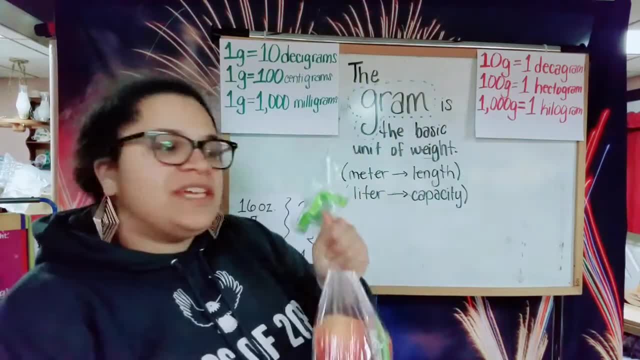 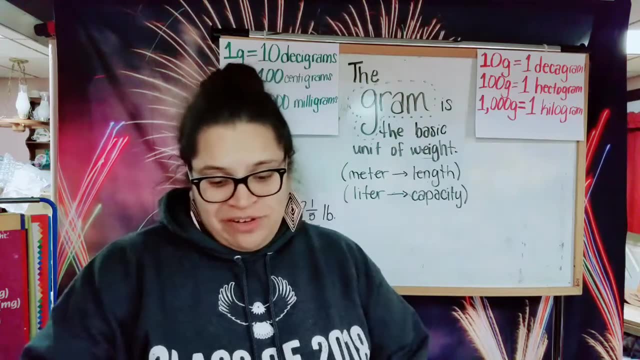 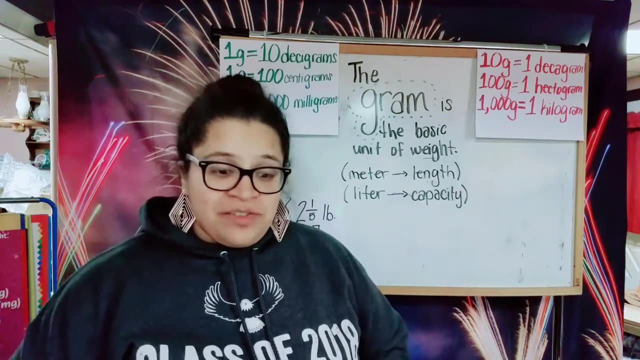 those bags of apples and see if you can kind of familiarize yourself with that measure of weight. So we see kilograms more than grams in the grocery store, but we do see those on all of our labels for the most part when we're shopping. And then the next unit we're going to talk about is way. 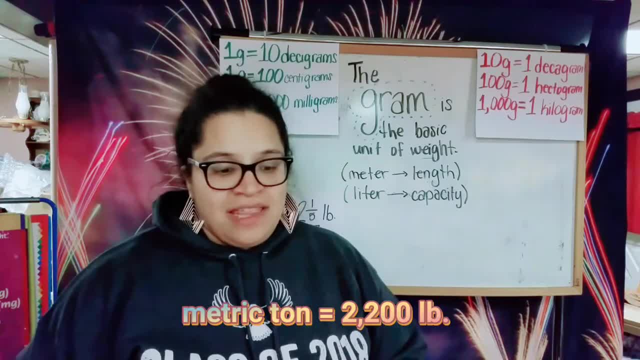 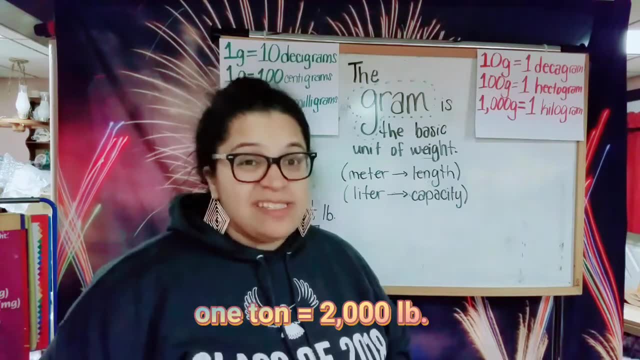 bigger than all of these. It is the metric ton, The metric ton. So we know that a ton is 2,000 pounds and we use tons to measure, like cars and boats and big, big, big, big, big, big, big items. So the metric ton is actually even bigger than that. The metric ton is approximately 2,200 pounds. Metric ton is 2,200 pounds, So is the metric ton bigger or smaller than the standard ton? That's right, The metric ton is bigger. It's 200 pounds bigger. 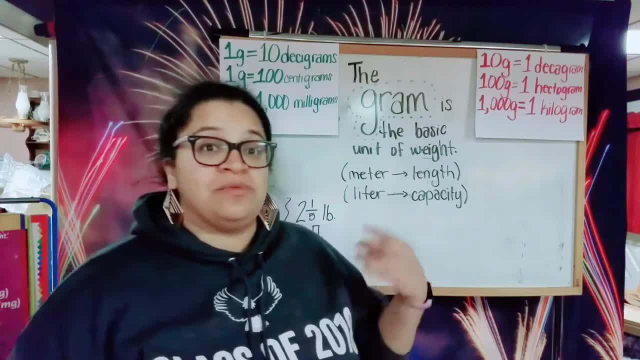 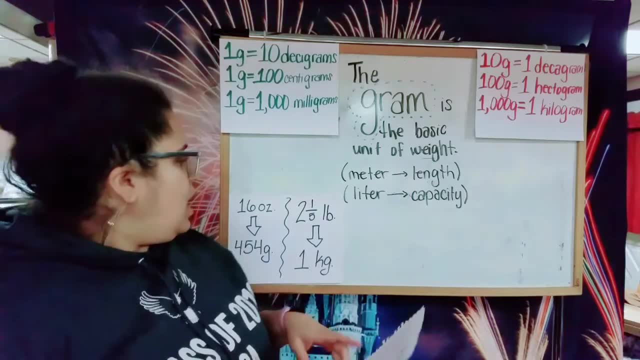 So, like I said, we use the same metric prefixes when we're talking about grams. So let's do some true or false, Okay, And I'll move out of the way so you can see. Oh yes, I'm sorry, I forgot, I had another. 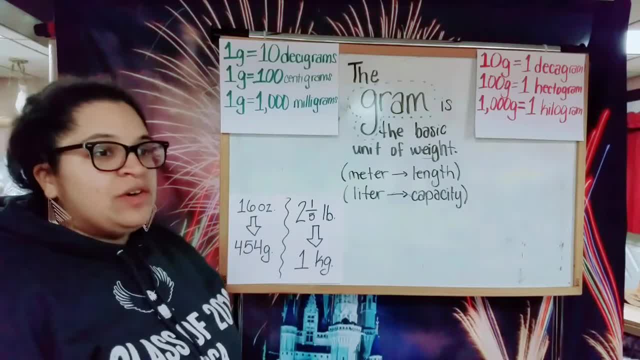 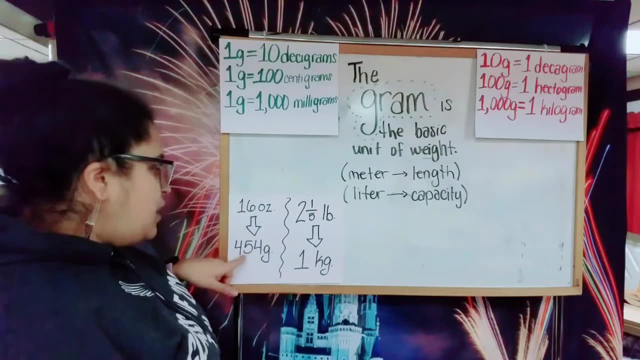 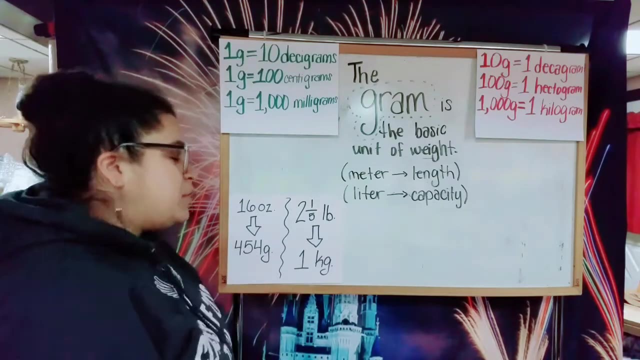 little bit of helpful hints here. So 16 ounces- We know that 16 ounces is two cups. 16 ounces is maybe a standard box of cereal. That is 454 grams. So if you shake your box of cereal up, if it's kind of full, that's about 454 grams. And then again, one kilogram is about two and one. 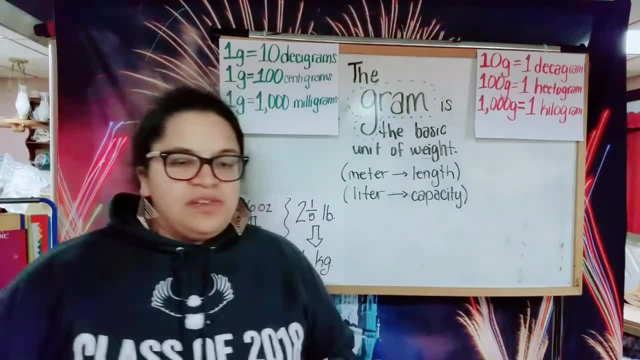 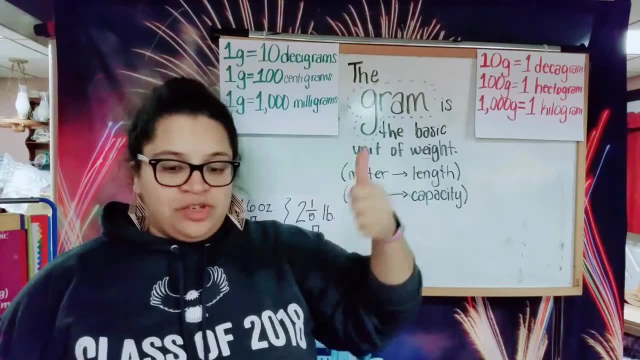 fifth pounds, All right. So let's go ahead and do some true or false. I will thumbs up for true, thumbs down for false. Why don't you do that with me? So thumbs up if it's true, thumbs down if it's false. 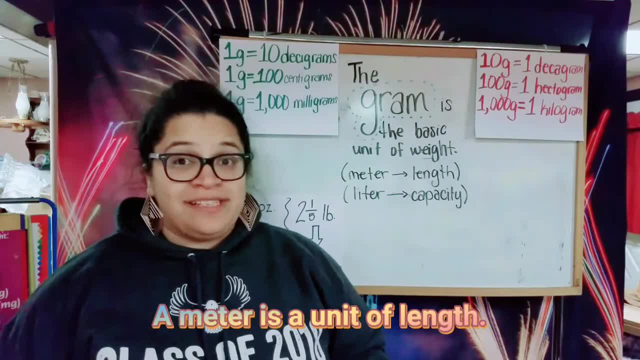 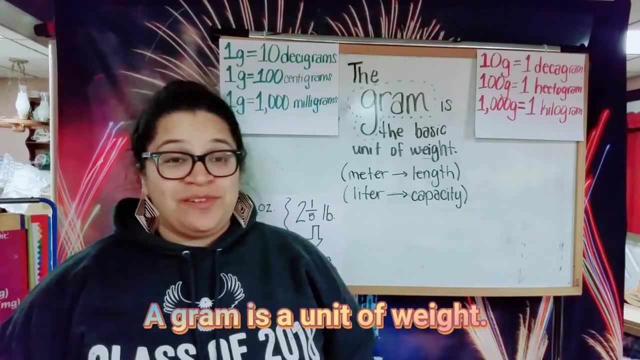 Firstly, a meter is a unit of length. Is that true or false? Meter is a unit of length- True. A gram is a unit of weight- True or false? True, Good job scholars, You guys are doing great. A meter is a little longer. 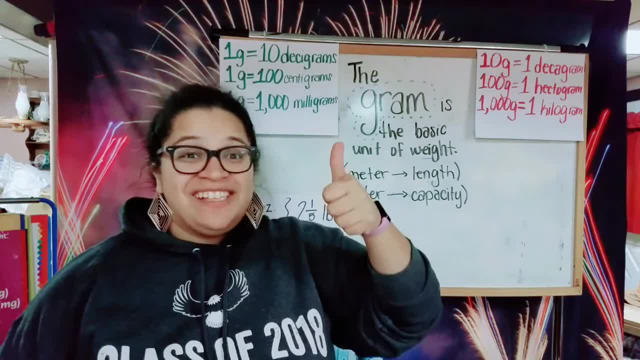 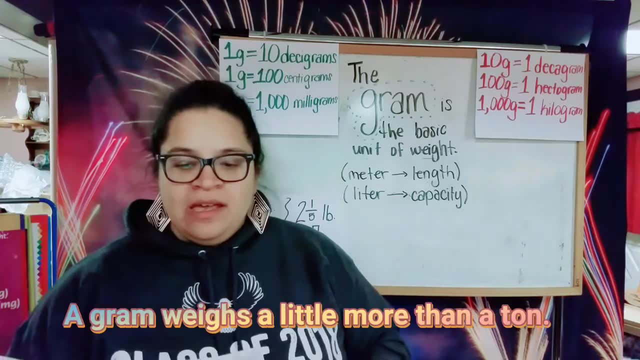 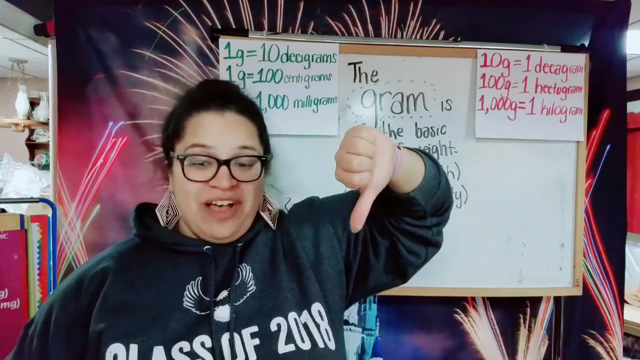 than a yard, True or false. True, That's right. A meter is about 39 inches And my yard is 36 inches. Good job, scholars. A gram weighs a little more than a ton. That's false. A gram is a really small unit of. 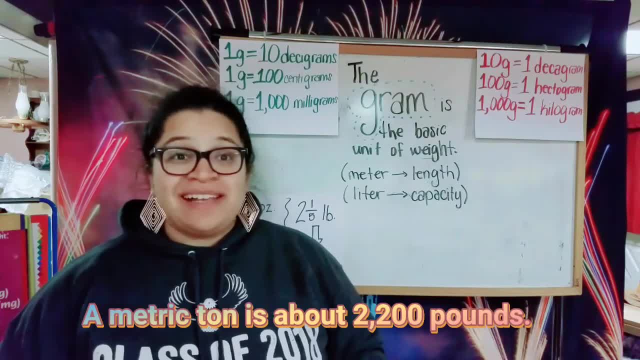 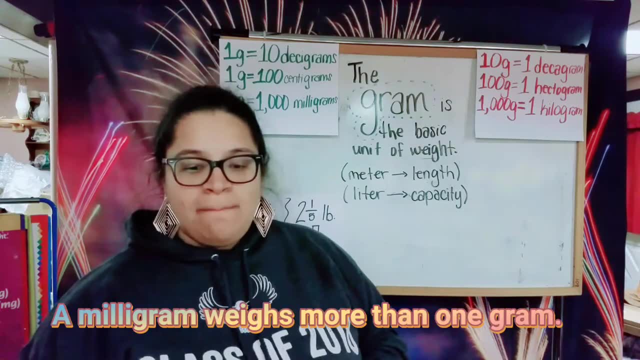 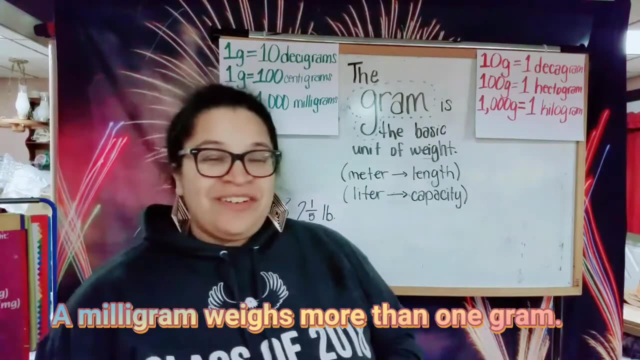 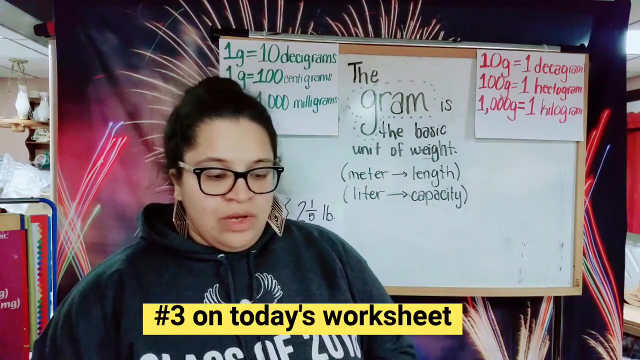 measure: A metric ton is about 2,200 pounds. True, Good job. And one more: A milligram weighs more than one gram. That is false. A milligram is actually one one thousandth of a gram. All right, Let's do one more exercise. 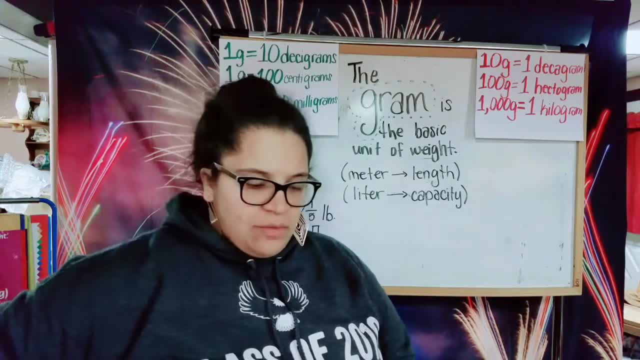 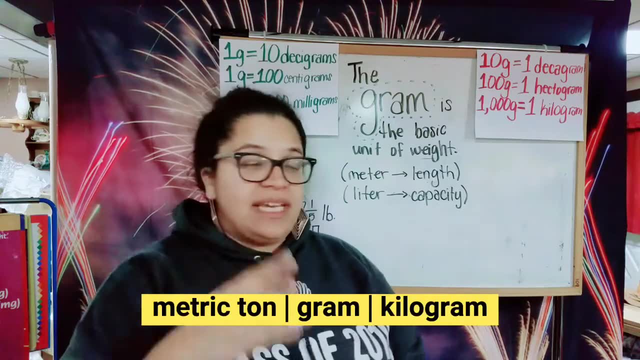 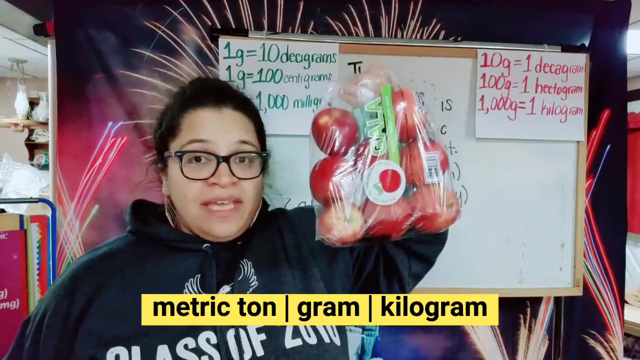 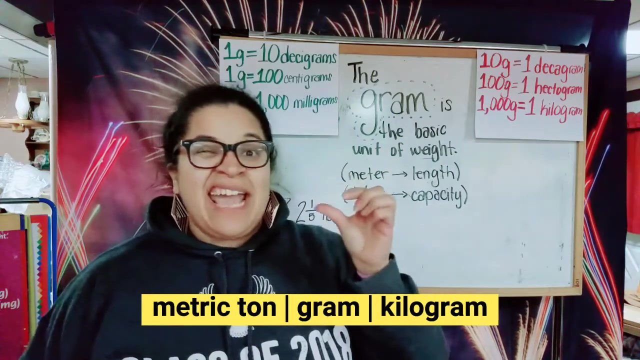 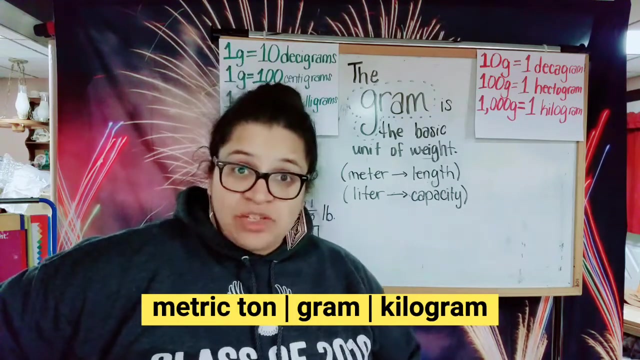 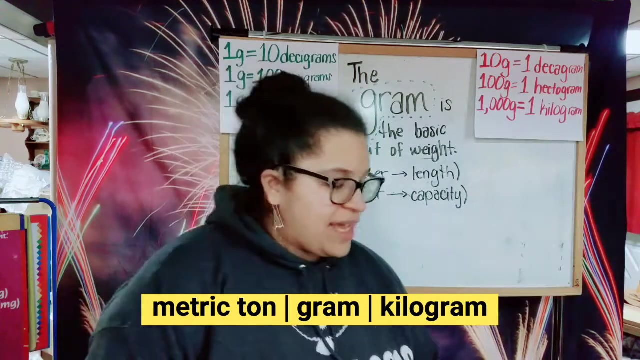 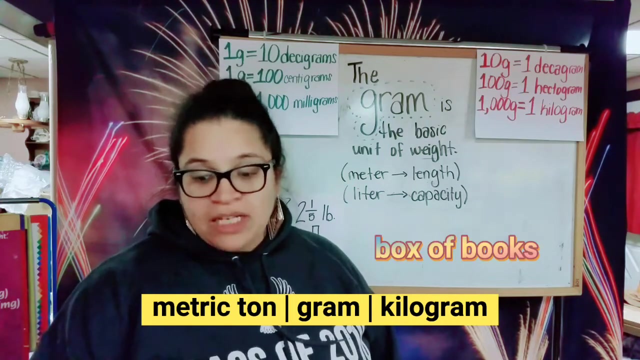 Let's see Which unit of weight would you use to measure these items. So you've got three options: A metric ton, a gram or a kilogram. So a metric ton is like a car, A kilogram is my bag of apples, And a gram I almost want to think of like a candy, a small candy size thing to measure a gram. So we're going to see which one of these we would, which unit of measure we would use for these common items. So medicine: Would you measure medicine in a metric ton, a kilogram or a gram Gram? Good job. What about a box of books? 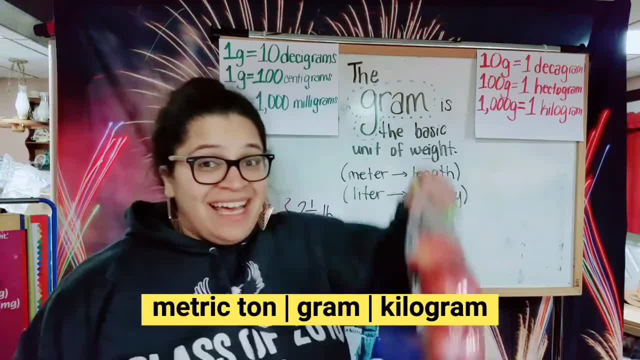 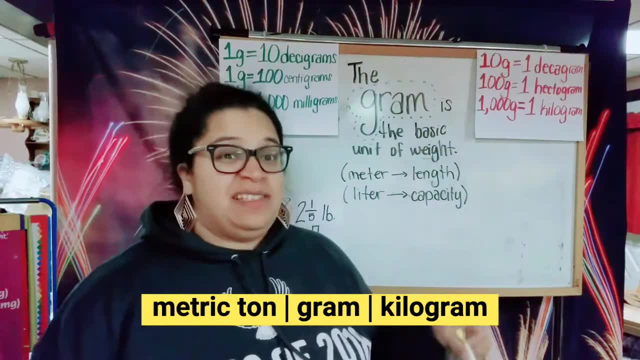 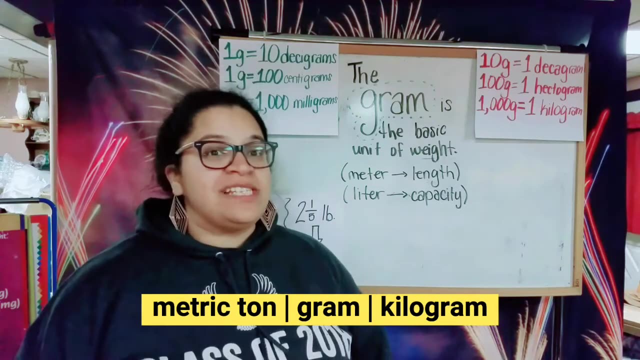 A box of books. Would you use a metric ton, a kilogram or a gram? I would definitely use a kilogram for that box of books. It's probably really heavy, Especially if it's hardcover books. let's see a house trailer. a house trailer. Maybe you've seen those getting pulled. 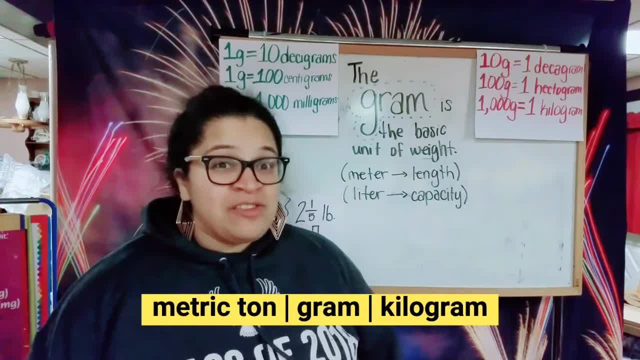 along on the highway as you're driving along with your grown-ups. A house trailer would use a metric ton which is 2,200 pounds a kilogram, which is about two and one fifth pounds or a gram or a kilogram of thelloar billion discrete extra volume. 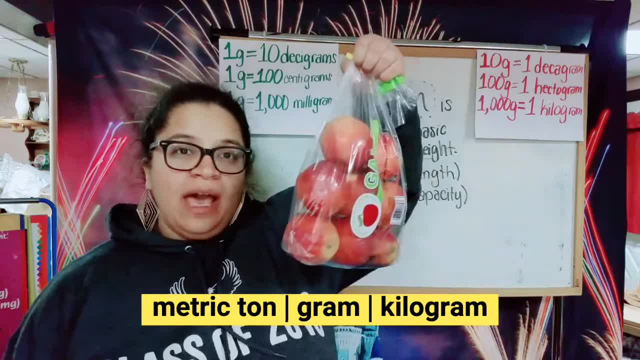 A house trailer would use a metric ton which is 2,200 pounds a kilogram, which is about two and one fifth pounds or a gram, A milligram Ch sneakily into the books. two and one-fifth pounds or a gram, which is really really little Metric ton. Good job. 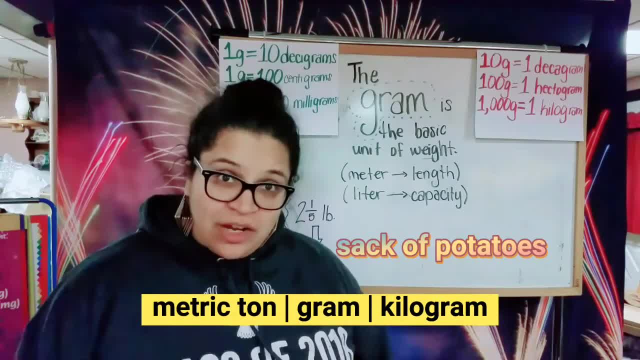 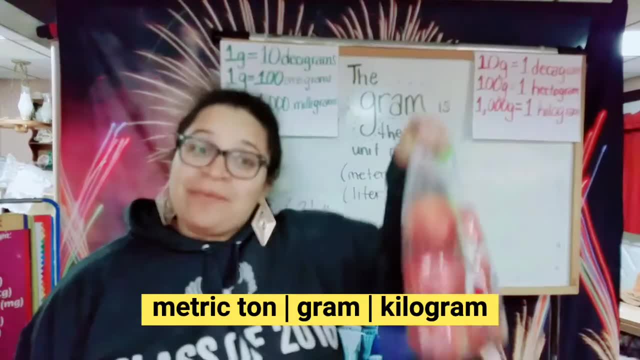 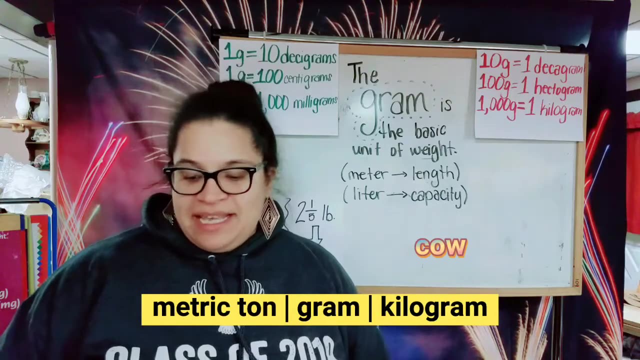 scholars, Let's do three more. A sack of potatoes? Oh, that's easy. I have one of those in my kitchen pantry. Would you use a metric ton, a kilogram or a gram to measure a sack of potatoes? A kilogram is right. Good job, scholars, And let's see A cow, A cow, A cow, Let's think. 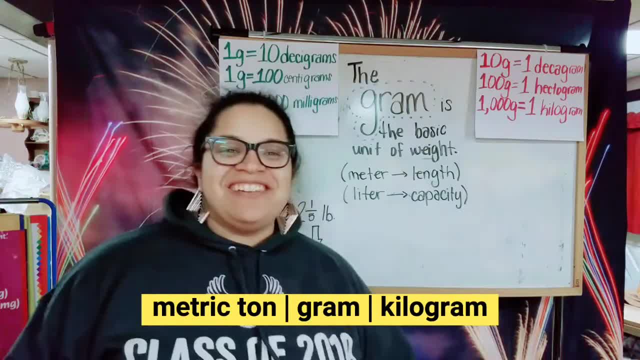 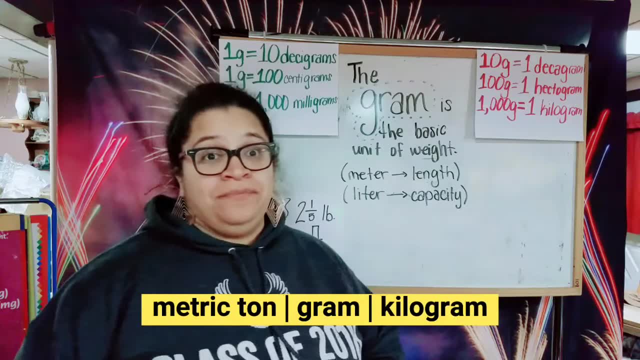 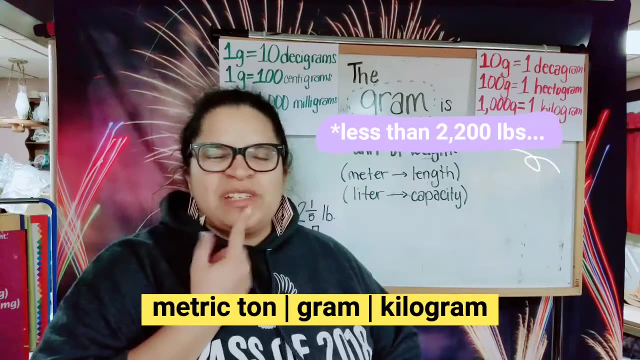 about it. Let's be a little reasonable here. Would we use a metric ton to measure a cow? Would we use a kilogram to measure a cow's weight, or a gram? Now, you might be tempted to say metric ton, but I'll tell you now: cows are less than a thousand pounds in weight, So we can't use a. 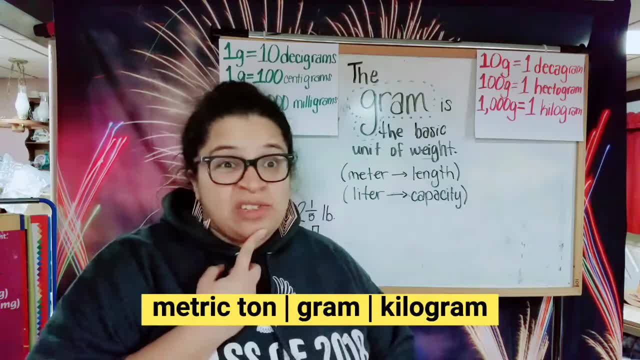 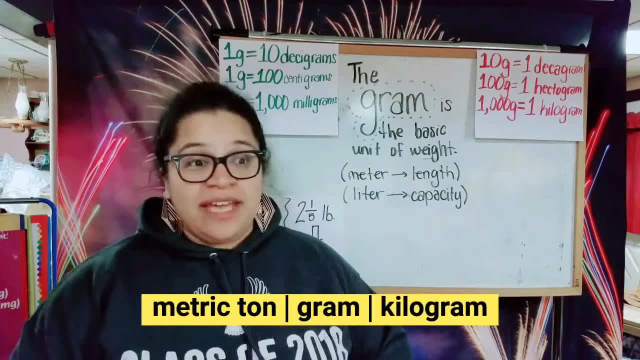 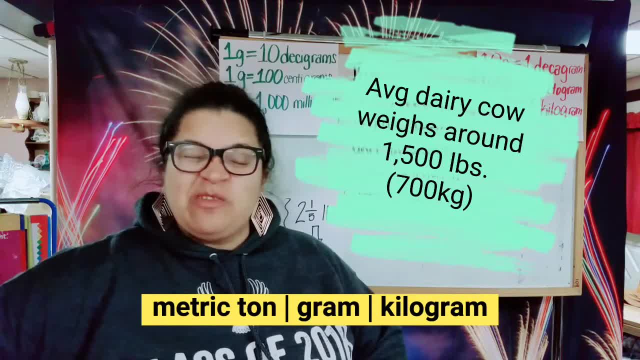 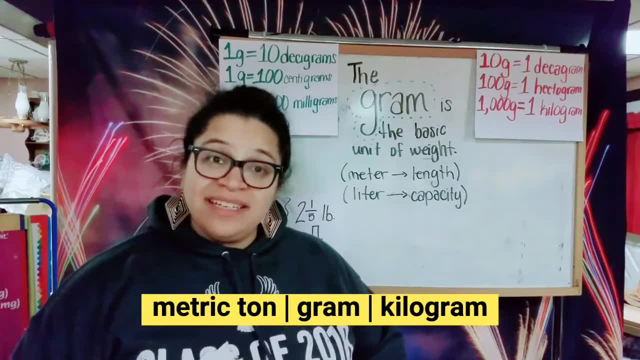 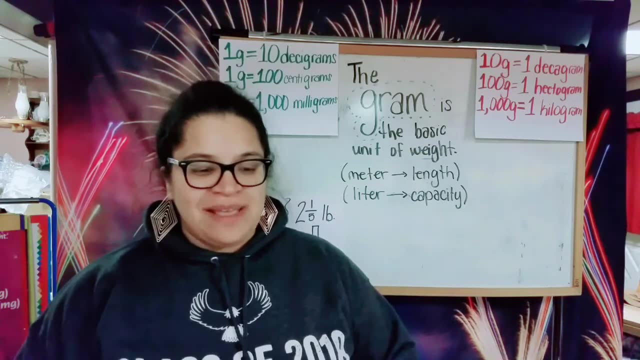 And let you know what the actual weight of a cow roughly is. And a ship, A ship that sails in the ocean. Metric ton. kilogram or gram. Metric ton. you've got it Good job. Thank you for sticking with me on this metric units of weight video. That's it for today. I'll go ahead and I'm going. 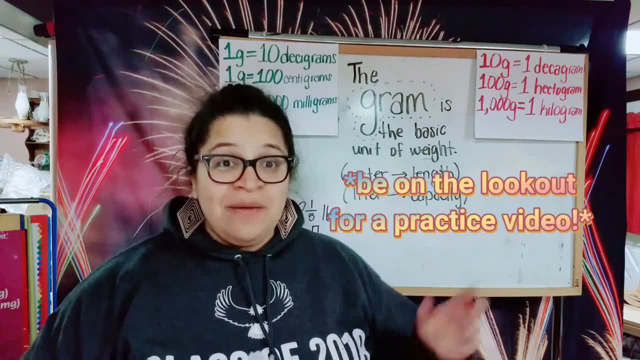 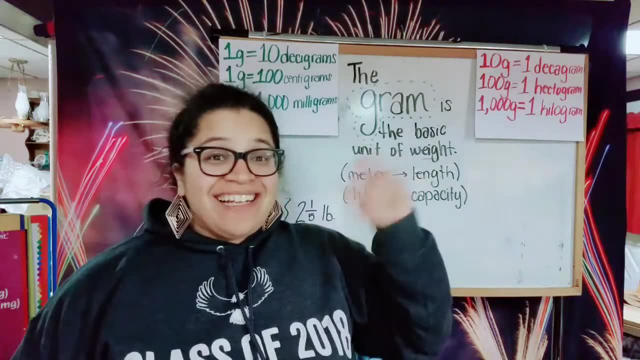 to put up another video of some practice problems from today's lesson, but I want to go ahead and sign off on this one. Thank you for watching. I'll see you next time. Bye-bye, Bye, scholars.